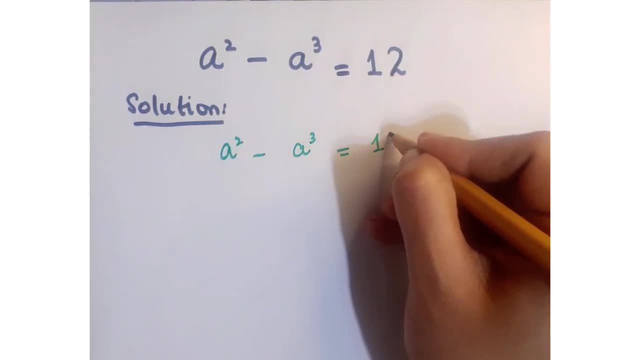 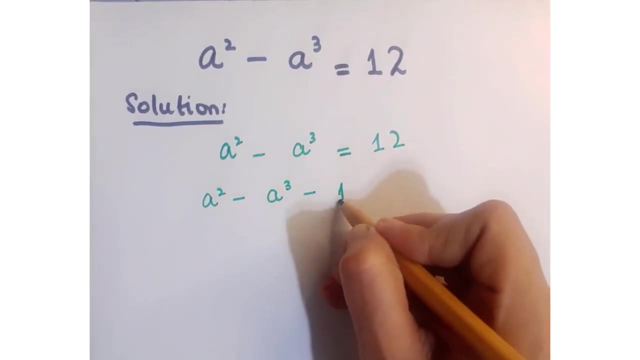 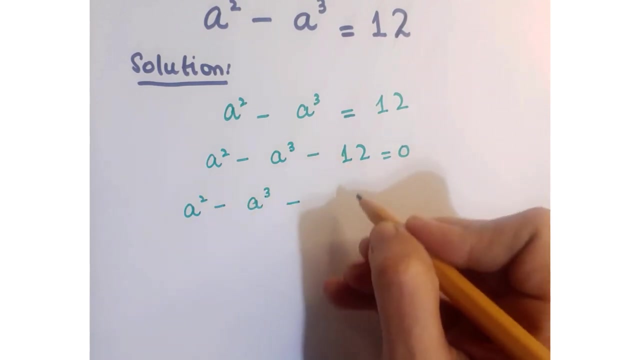 a square minus a cube is equals to 12.. First of all, move this 12 on the left hand side, So sign gets changed. Next, this is square and this is cube. Now you can split this 12 in such: 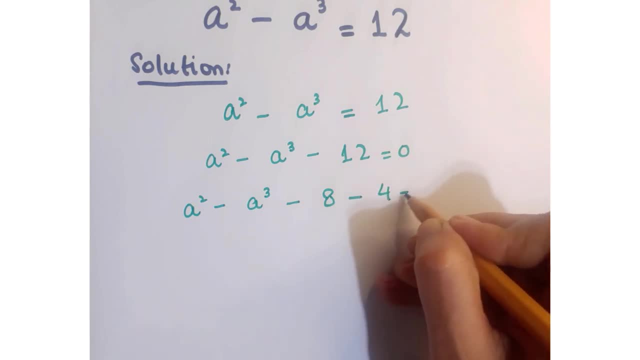 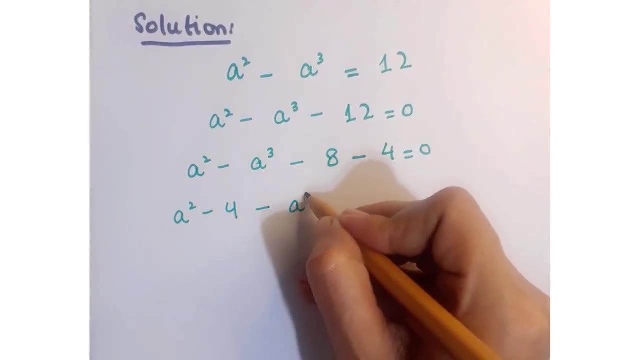 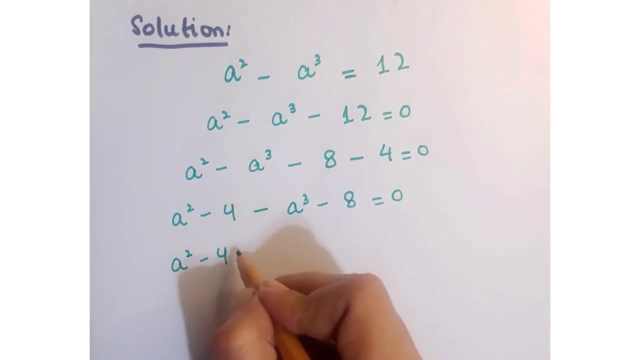 a way that 1 is like 8 is a cube of 2 minus 4, right Now, rearrange the equation as a square minus 2 and minus a cube minus 8 is equals to 0.. Further, you can write this as a square: This is: 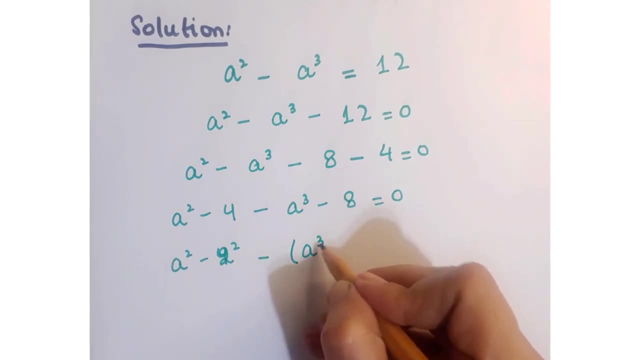 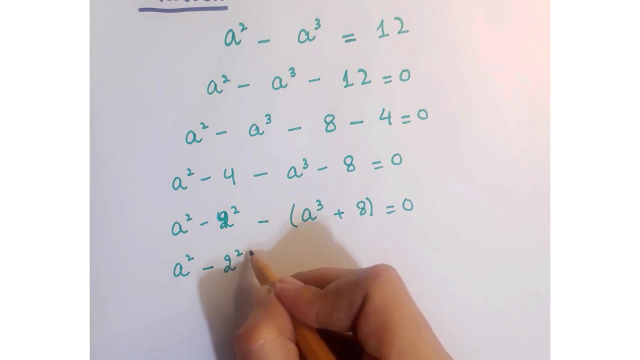 minus 2 square, taking out minus common. So we have a cube plus 8 inside the brackets. or you can write here: a square minus 2, square minus a cube plus 2 cube is equals to 0.. Now we are going to. 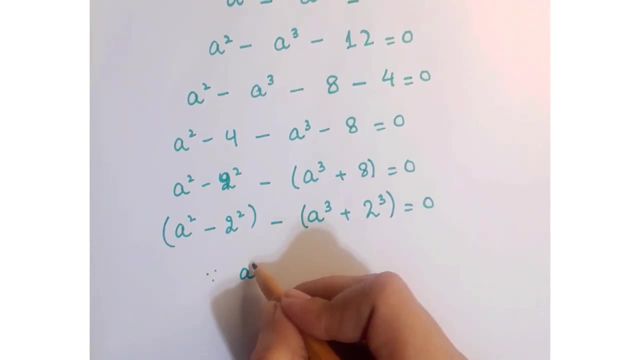 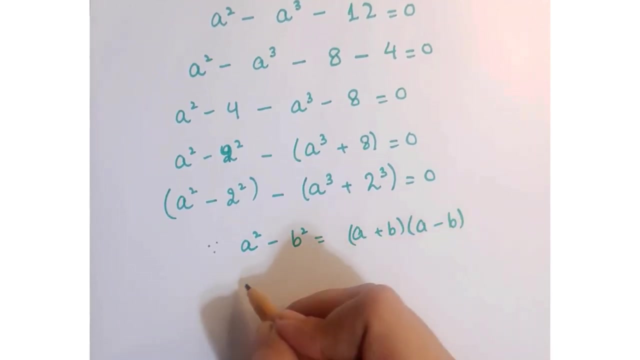 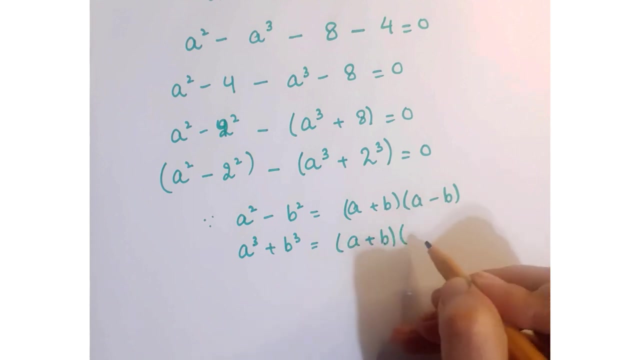 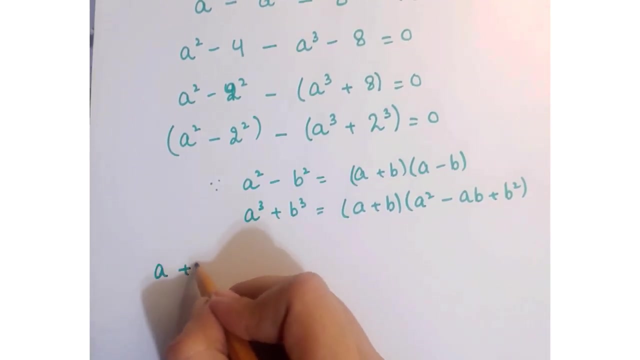 apply the algebraic identities here. First of all, a square minus b square can be written as a plus b into a minus b, and secondly, a cube plus b cube can be written as a plus b into a square minus ab plus b square. So here we are going to write a plus 2. 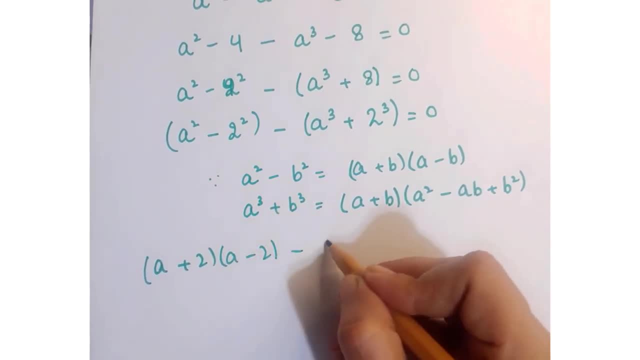 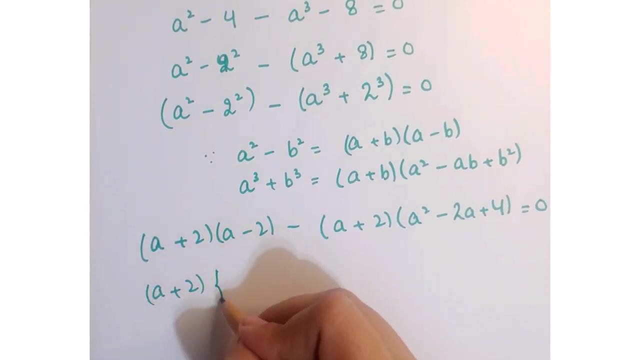 into a minus 2 minus This is a plus 2 into a square. minus 2a plus 4 is equals to 0.. Now, out of these two terms taking out a plus 2 common, So we have a minus 2 minus a square. minus 2a plus 4 is equals to 0.. 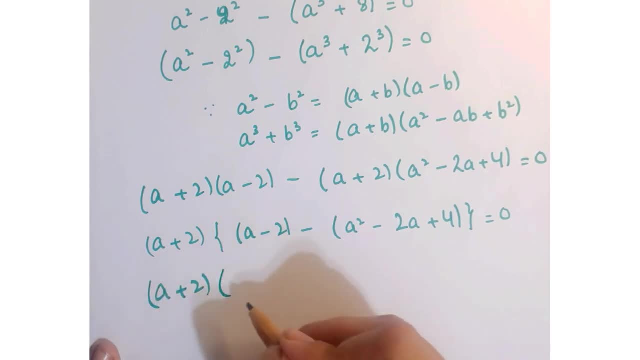 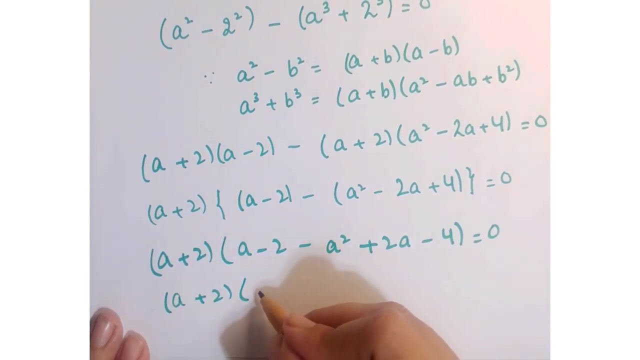 Next, this is a plus 2.. Here we have a minus 2 minus a square. This is a plus 2 minus a square. minus a square, minus 2a, plus 4 is equals to 0.. Or you can say: this is a plus 2.. This is a and this is 2a and this is minus a square. 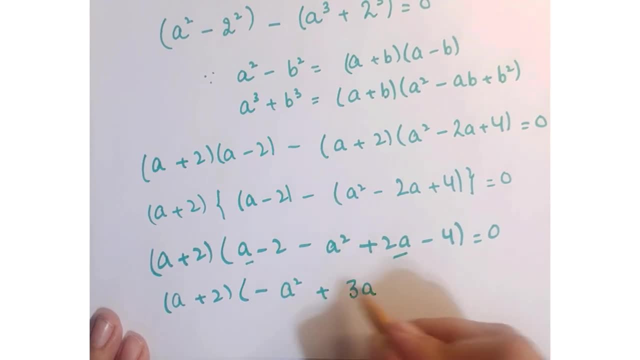 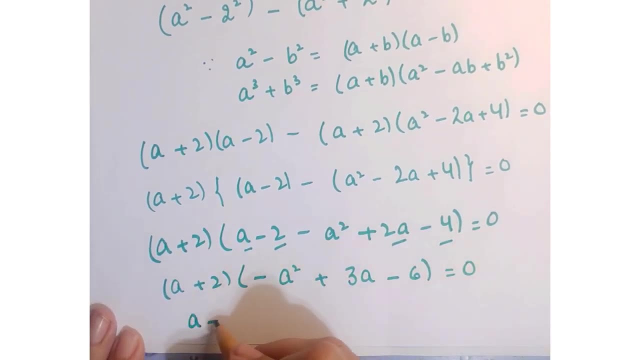 This is minus a square, plus this is 3a, and these are two constants, So minus 6 is equals to 0.. Now this implies a plus 2 is equals to 0 and this is minus a square Plus 3a. minus 6 is equals to 0.. 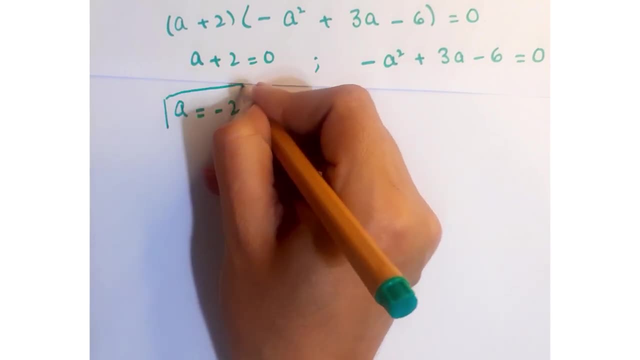 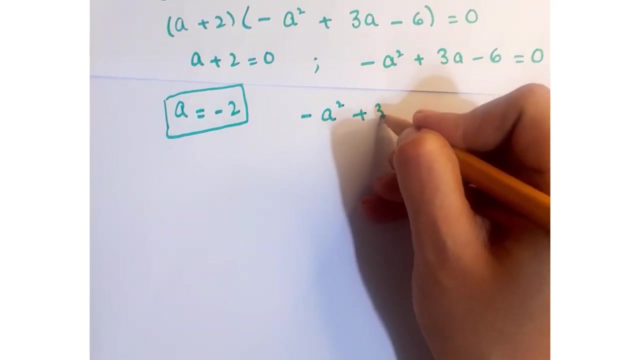 a is equals to minus 2, right, So this is one value of a. Now, this is a quadratic equation. This is minus a square, plus 3a, minus 6.. We are going to divide the whole equation with minus 1.. 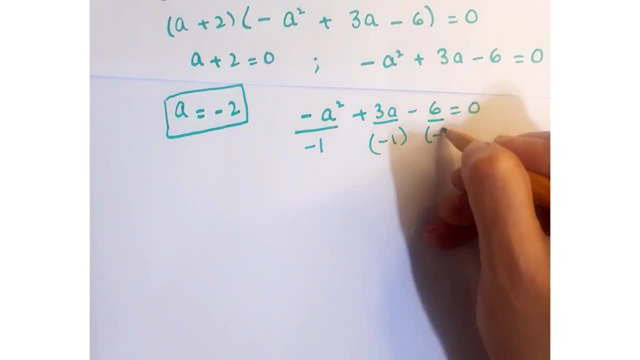 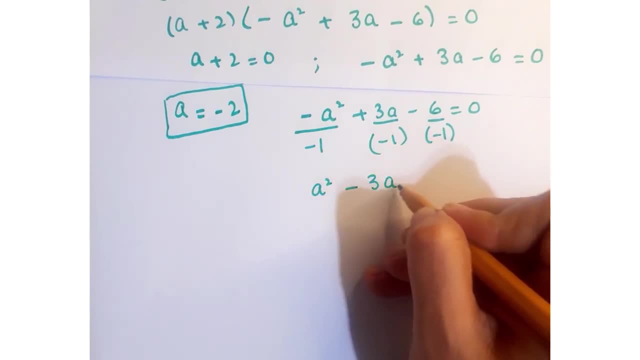 So we get here a square minus 6.. So we get here a square minus 6.. So we get here a square minus 3a. minus 6 is equals to 0.. In fact, this is plus 6, right. 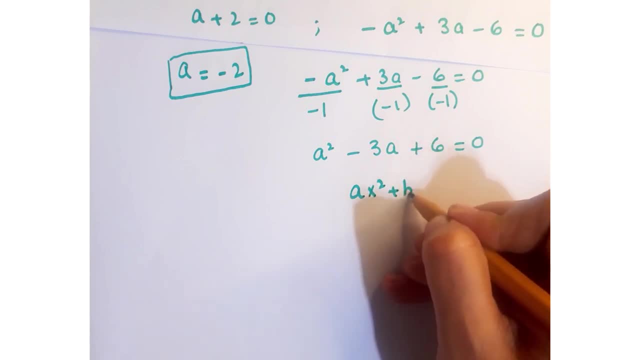 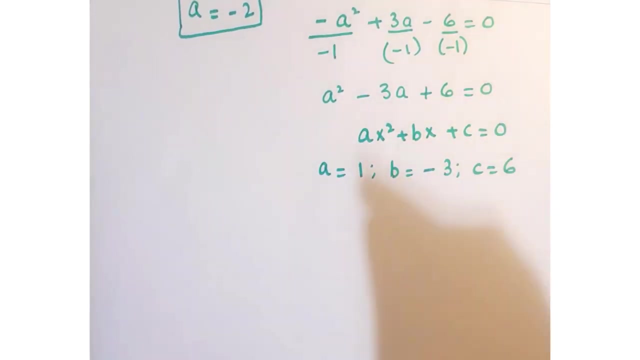 Now comparing this equation, the standard quadratic equation, that is a x square plus b, x plus c, is equals to 0.. So we have: a is 1, b is minus 3 and c is equals to 6.. Now applying this equation, we get here a square minus 3a minus 6.. 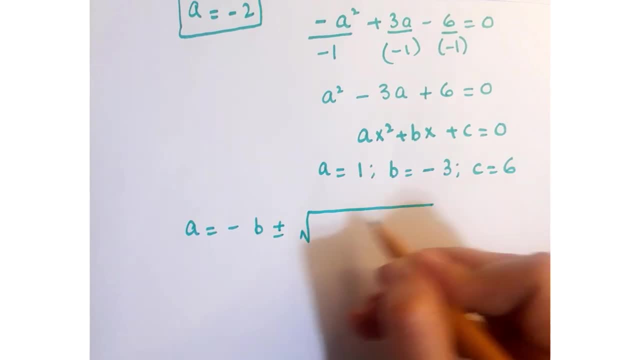 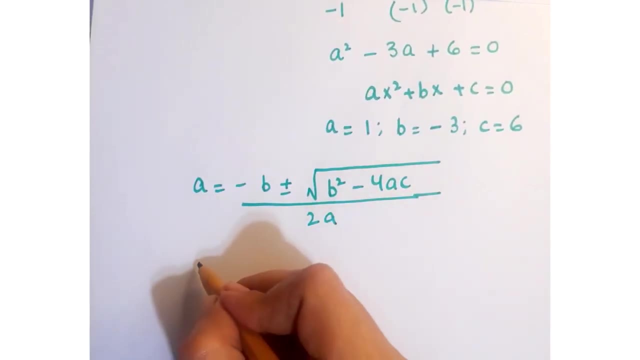 So we get here: a square minus 3a minus 6 is equals to 0.. Now the quadratic formula plus minus, this is under root b square minus 4ac upon 2a. So we have a is equals to. 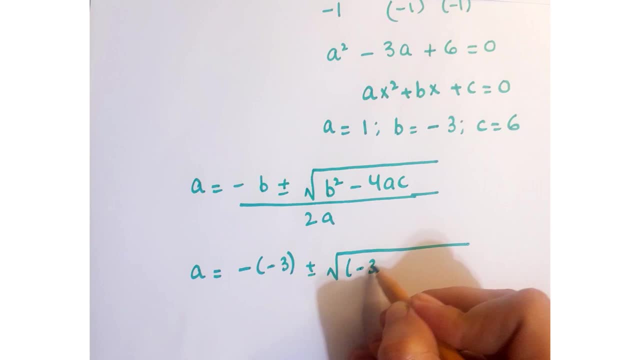 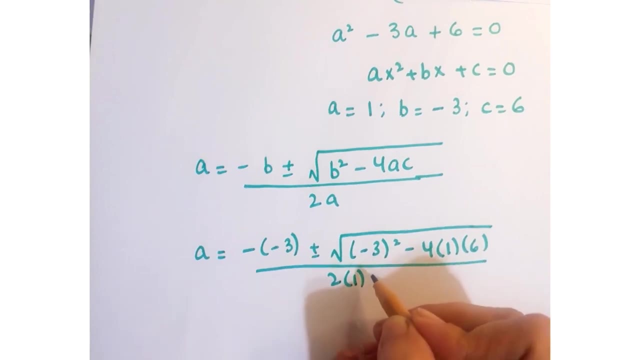 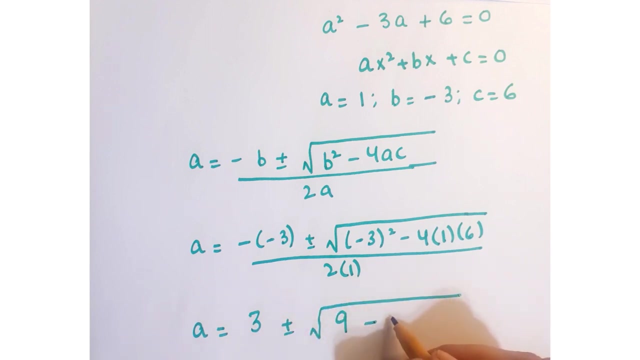 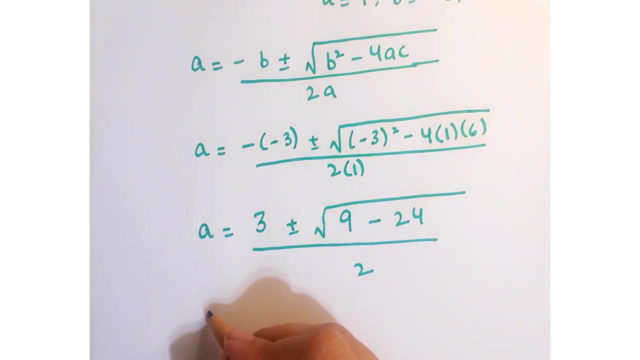 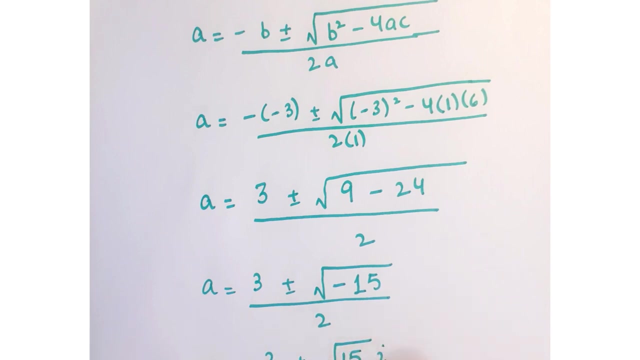 upon 2 into 1.. Further, you can write here: this is 3.. minus 9 minus 24 upon 2. or you can write: a is equals to 3 plus minus. this is minus 15 upon 2. further, the a is equals to plus minus 15 I upon 2. so these are. 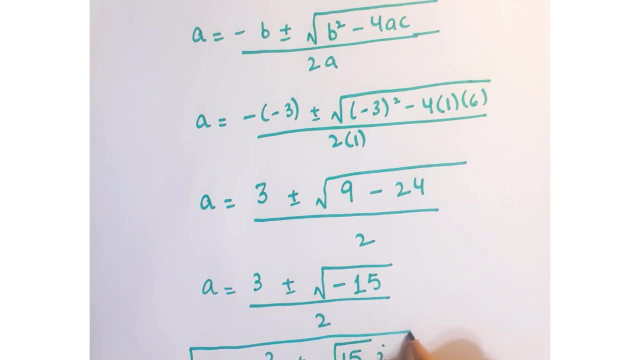 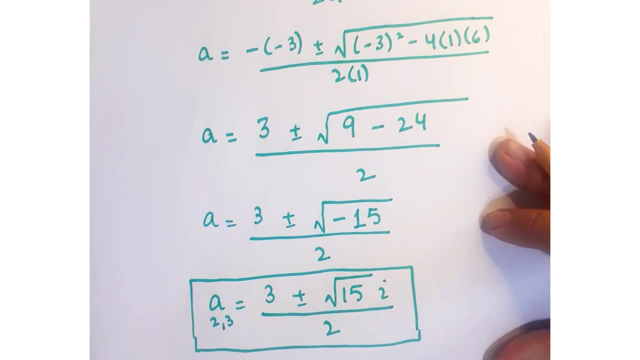 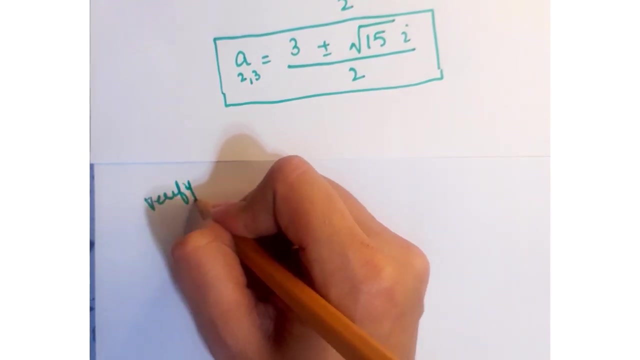 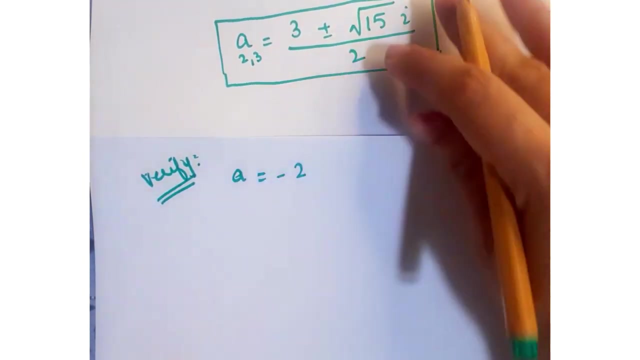 the second and third are the complex roots of this cubic equation. so we are going to check the real root, that is, verify. a is equals to minus 2 for this equation. the equation that we are given is a squared minus a cube is equal to minus 2.